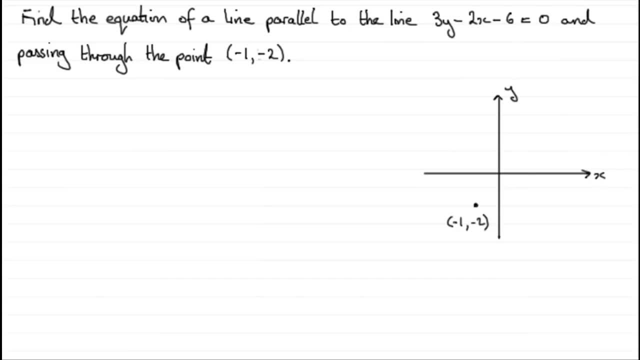 I could do it is to write it in the form: y equals mx plus c, Because when it's in this, because when it's in this format, I can see which way it slopes and also where it crosses the y-axis given by the number or constant C. so let's start by 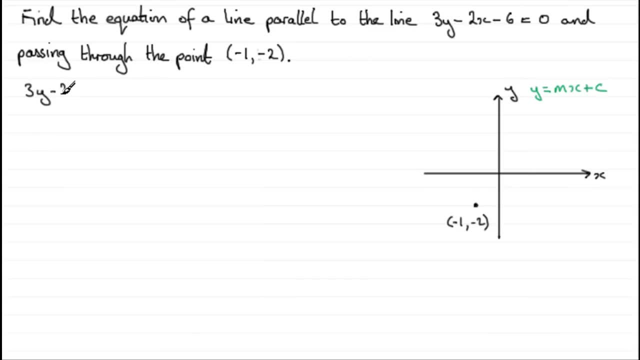 taking our line 3y minus 2x minus 6 equals 0 and to get it into this format I need to first of all add 2x and 6 to both sides, to give me 3y equals 2x plus 6. now I'm going to get rid of that 3 by dividing both sides by 3 and I get y. 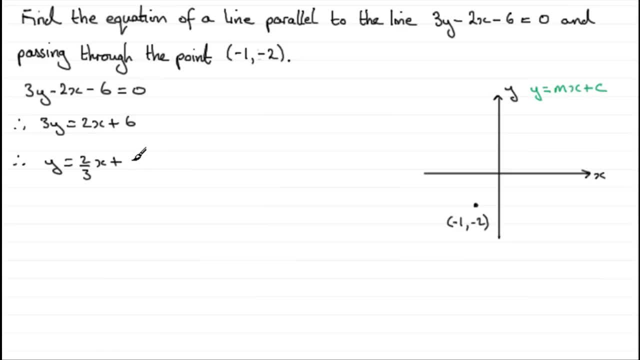 equals 2 thirds x plus 6 divided by 3, which is 2. so I can clearly see now that this line has a gradient of 2 thirds and when x is 0, y is 2, which will tell me that it crosses the y-axis at 2 units. 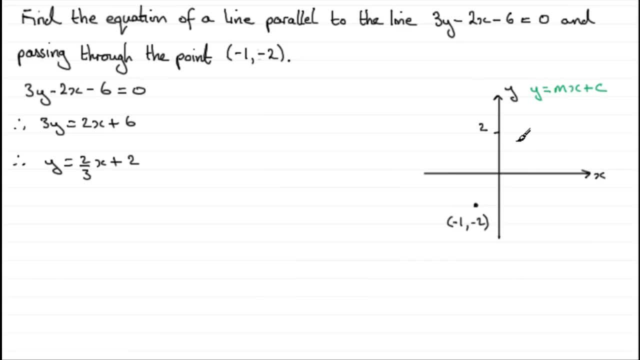 up. let's say that's the point where y is 2. so a gradient of 2 thirds is going to be a line coming through the 2, something like that, a positive gradient. so what I'm looking for now is a line passing through minus 1, 2, which is parallel. so 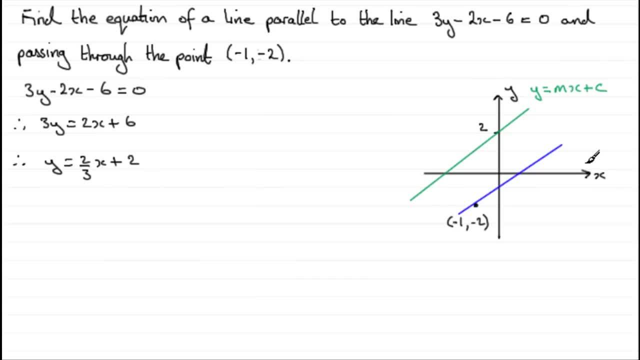 that line is going to look like this, something like that. so how do I get this line? well, I've got its gradient because it's parallel. now the gradient is 2 thirds. the M value, if you like, is 2 thirds. so if that's the case, I might as well use y minus y. 1 equals M. bracket x: 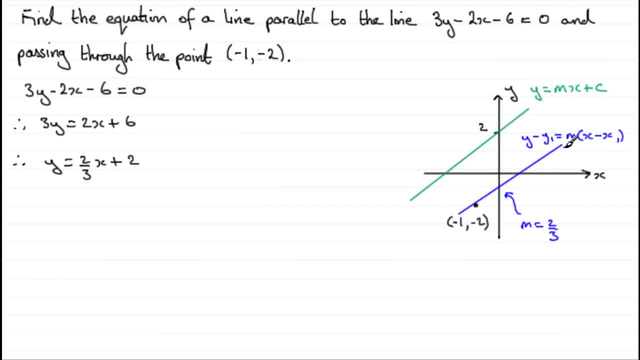 minus x, 1 as the form of the equation of this line, because I've got M x, 1, y, 1 is just a point on the line and I've got that point here. it's minus 1 minus 2, so I'm in a position to get the equation that. 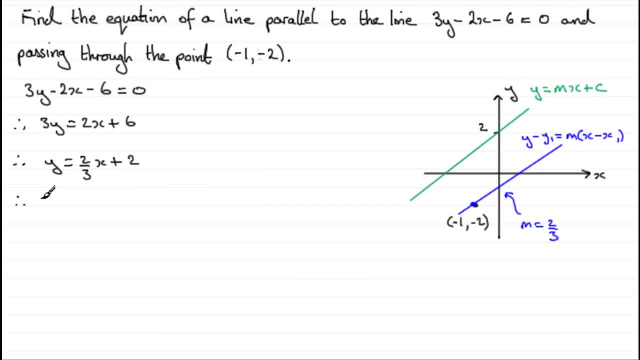 line, so let's just write an intro here. therefore, the equation of the line, say the parallel line of the parallel line, okay, is what is it going to be to be? what is going to be? y minus y1 being the minus 2 equals M being the 2. 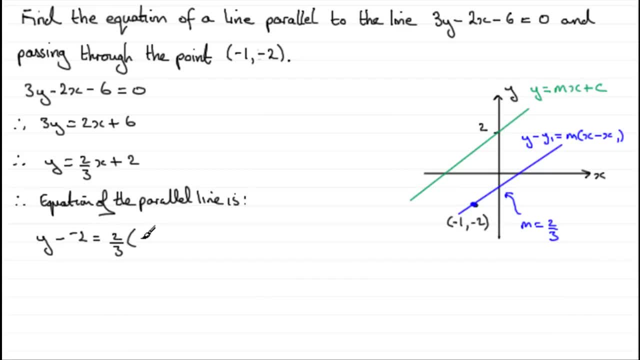 thirds, bracket X minus X 1. X 1 is the minus 1, so that's essentially the equation of the line. depending on the question, I would write it in certain formats. suppose we're going for y equals MX plus C format. I'd most probably want to multiply by 3 and I would times both sides by 3 and get 3y. 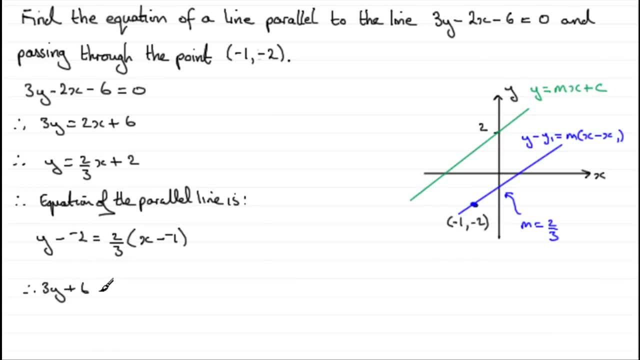 here. this is plus 2, so we end up with plus 6 equals. if I times this side by 3, the 3 will cancel and just leave me with 2 times X plus 1, which would give me 2 X plus 2. so if I was to subtract 6 from both sides, I'd have 3y equals 2x minus 4, and 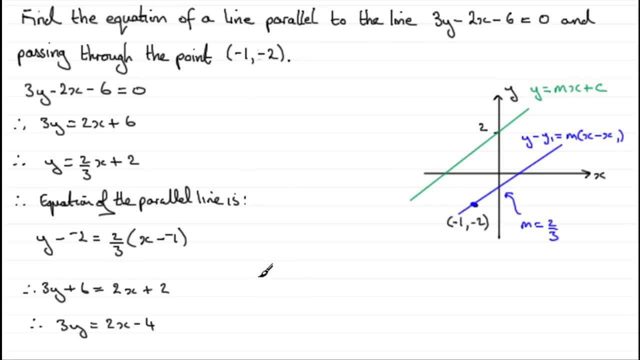 then finally to get the equation of the line, we would therefore have y equals. if I divide both sides by 3, 2 thirds, X minus 4 thirds, and you can see it's got the same gradient- 2 thirds. and where it crosses the y-axis, when X is. 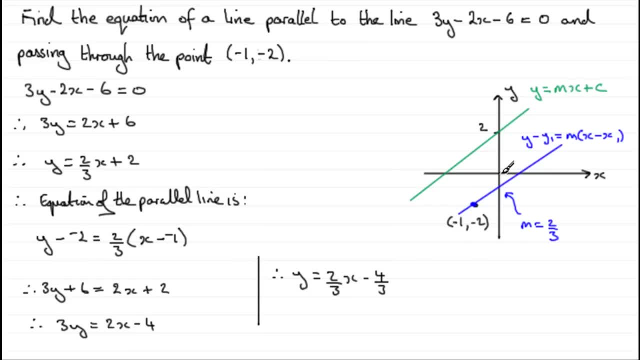 0 is at minus 4 thirds and, okay, it's not accurately drawn, but it's not too bad. it gives us an idea that it looks reasonable. okay, well, I hope that's given you an idea, then, how to do examples like this one. and that brings us now to the 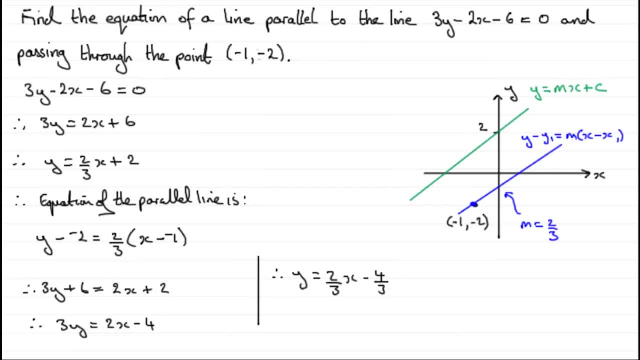 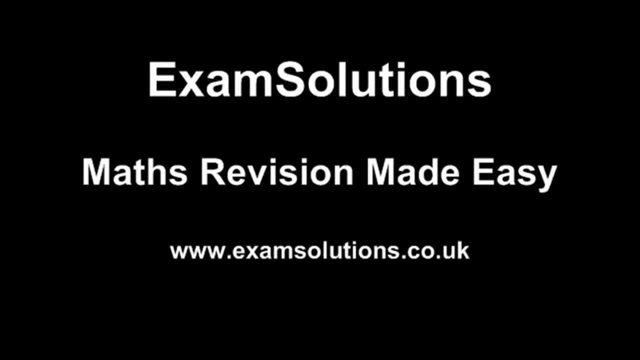 end of this particular example, you.